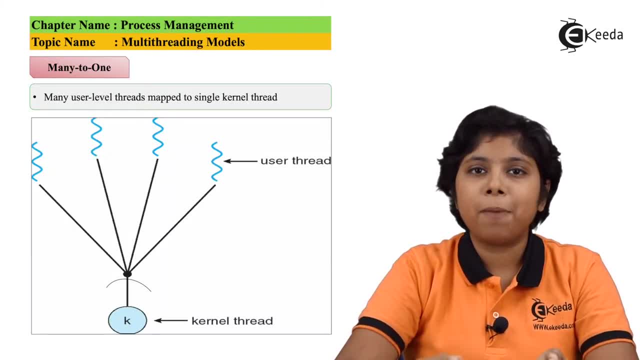 one model. there are many user level threads mapping to the user only kernel level thread. now, as thread management is done by the thread library at user space, it is more efficient, however, and the entire system will get blocked if only a single thread is making a blocking system. 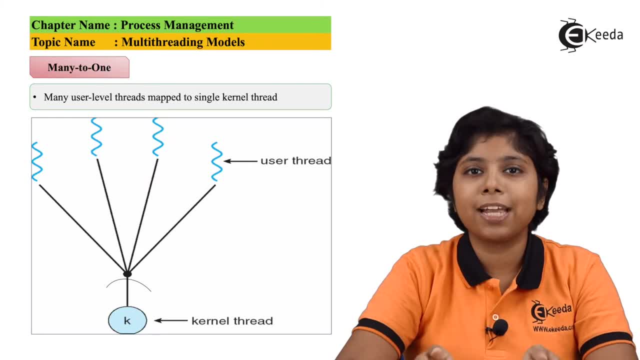 call and also all the user threads cannot run concurrently, as only one kernel thread can be executed with one user thread at a time, so the other user threads must wait for the user threads to be mapped with the kernel green thread, which is a thread library provided by solaris 10. 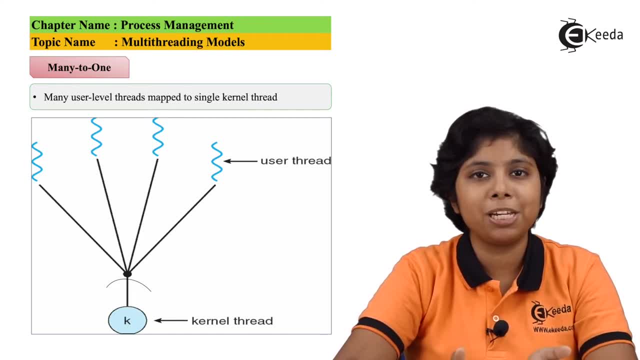 and the older version of the solaris 10 with the linux family 2 are used as one-to-one model implementing their operating system. the early versions of java also use this green threads. now, as there are discrepancies of not using the threads concurrently and other challenges this. 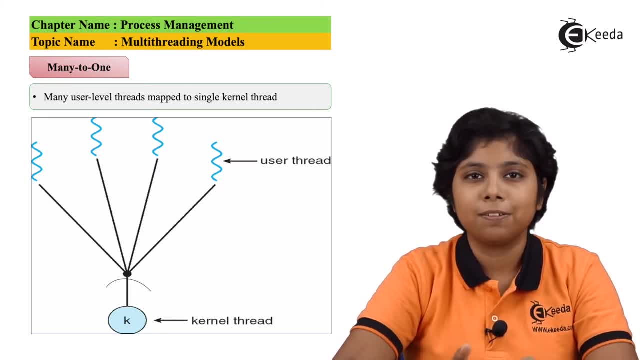 many-to-one model is not implemented nowadays. now the next model is a one-to-one model. in one-to-one model a single user thread is mapped to a single kernel thread. here all the user can run concurrently with the help of each kernel corresponding to them, and also a kernel can call any other thread if a thread cause a non-blocking and blocking system. 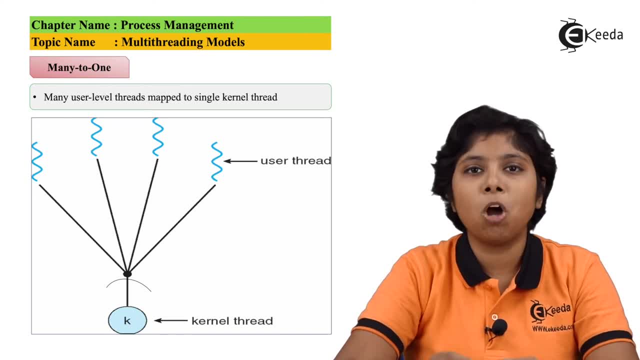 call now. the system will not get blocked at all. the only drawback in this one-to-one system or model is that using and creating the user thread will also cause the using and creating a separate and corresponding kernel thread too. so the overhead of this kernel thread thread creation can be a burden on the system's improvement. 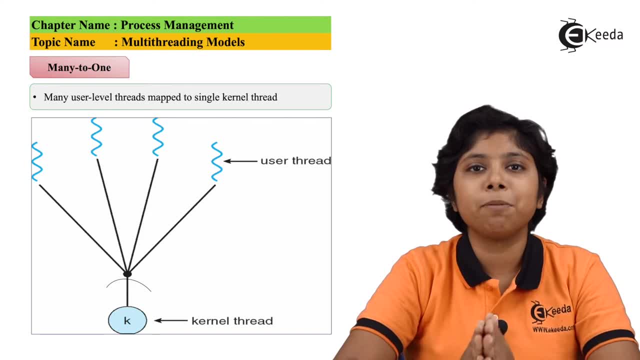 better performance. Now this performance can be done with the help of restricting the number of kernel threads supported by a system. Now, many models and many cooperating system implements this one to one model, But because of the drawbacks, many users restricting it to the Linux along with the Windows. 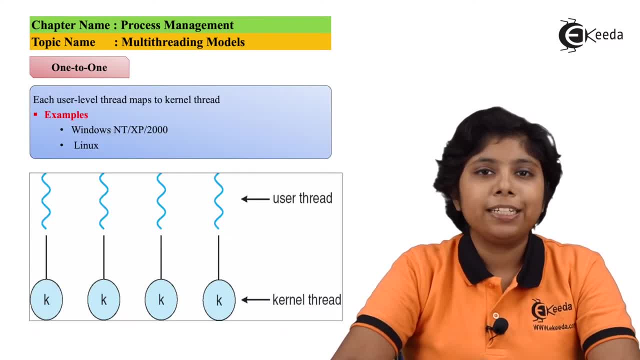 families use this one to one model. The third part is a many to many model In a many to many model. it multiplexes the many user level threads to be mapped with equal or lesser number of kernel level threads. Now this kernel level threads can be. 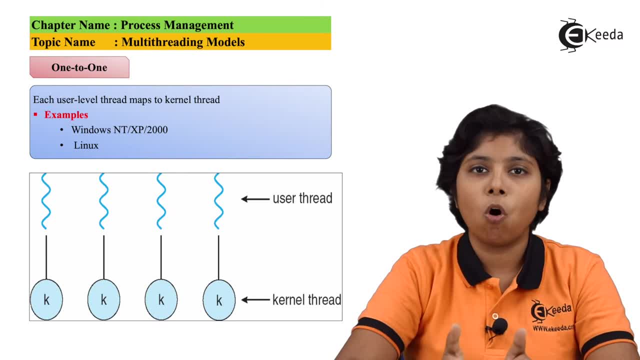 implemented directly via an application or depending on a machine. An application may be allocated more kernel level threads on a multiprocessor rather than a single processor. Let's consider the effect of concurrency on the systems Where a many to one model, the many user level threads, cannot run concurrently as one kernel. 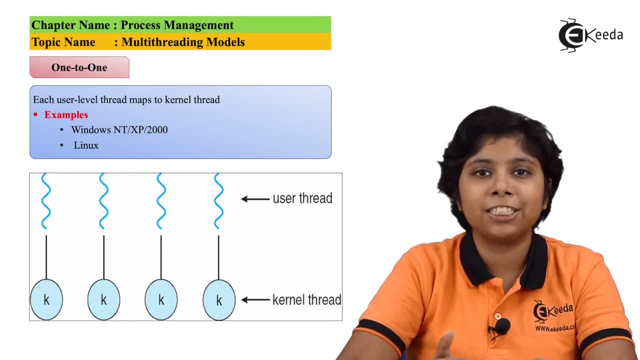 level thread can execute an user level per at a time And in one to one model. this can be done because an user level thread is supported by its corresponding kernel level thread, But the incurring overhead of the creation of kernel level thread is there So many to many model supports none of these. 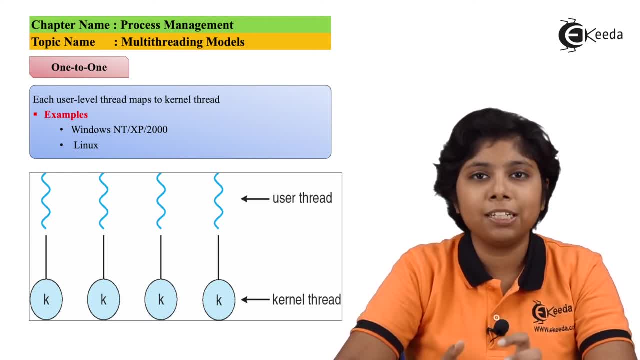 efficiencies. Now, these discrepancies can be done with the help of this many to many model. In many to many model, many user level threads can be created by a user where it can be supported by the kernel differently. on this, multiple processors, Now the multiple processor, and in each core. 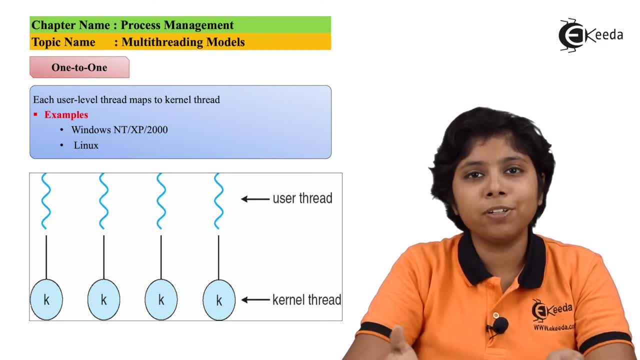 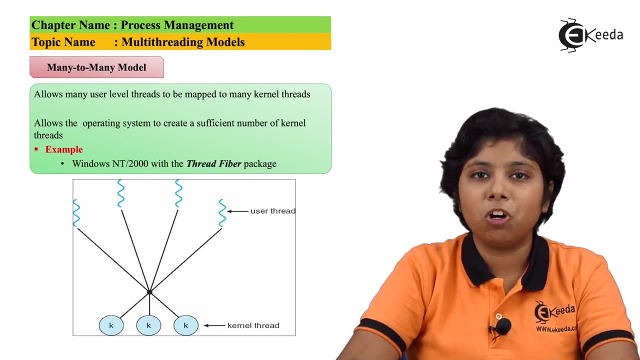 this, each kernel can be executed And also it can be run concurrently, so the concurrency problem is also solved. If thread is making an block system call, then other threads in the user spaces can perform the kernel level threads to execute the actual function. Now one variation of the many to many model that it includes the user. 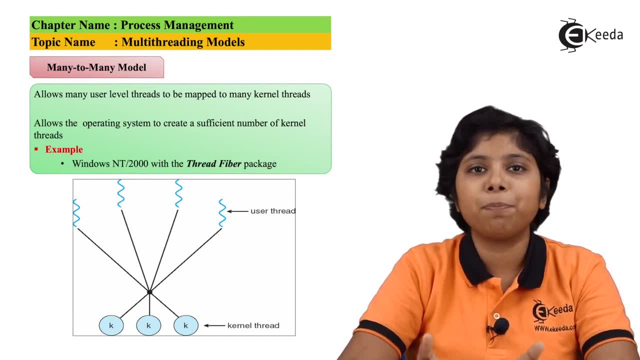 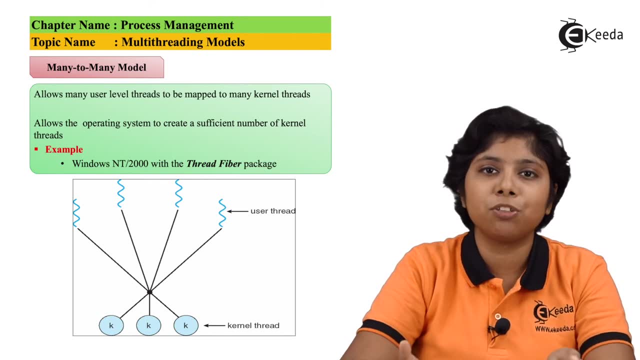 level. many user level threads can be mapped to equal a lesser number of the kernel threads, along with each user level thread can be corresponding to each kernel level thread. this level or this model is known as a two-level model. this two-level model is often implemented in many operating systems. as it can be performed, the advantages.